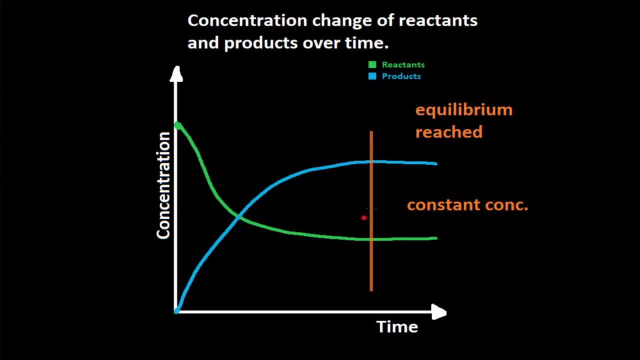 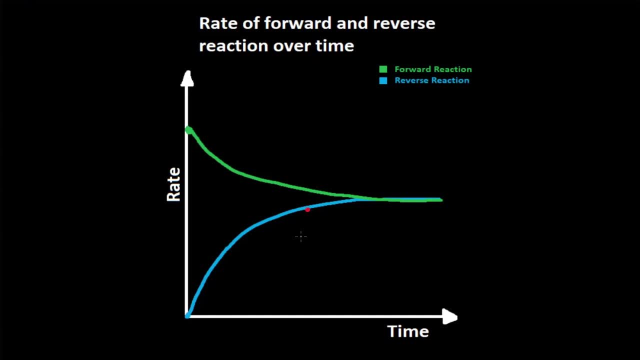 are at constant concentration. Basically, when the lines turn straight, equilibrium is reached. Rate of forward and reverse reaction over time. So when do you think equilibrium is reached? You remember dynamic equilibrium means the rate of the forward reaction is equal to the rate of the reverse reaction. This means equilibrium is reached when they are both equal to each other. 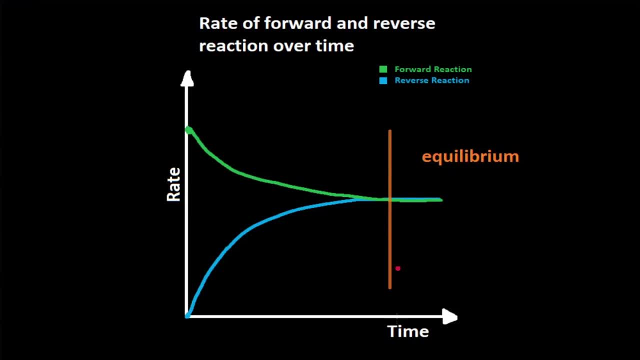 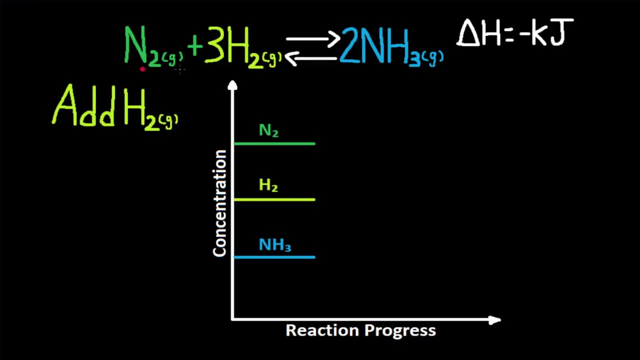 Basically, when the lines turn straight, equilibrium is reached. If H2 is added to this reaction, describe the effect on the graph. So, if H2 is added, don't point at what is being added. so this is a shift right. A shift right points at the product, so the products increase, and it doesn't point at 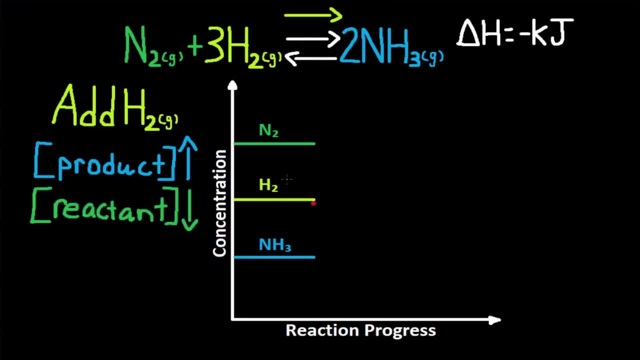 the reactants, so the reactants decrease. To graph it, it's as simple as graphing what we described. H2 is added, so H2 increases. H2 is a reactant and reactants decrease, so H2 decreases. however, it won't decrease more than its initial amount. N2 is a reactant and reactants decrease, so N2. 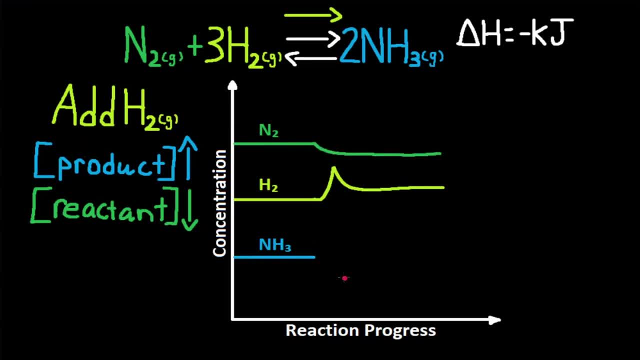 decreases. NH3 is a product and products increase, so NH3 increases. Now the impact of increasing and decreasing is dependent on the coefficient. so H2 has a coefficient of 3, so it would decrease more compared to N2, which has a coefficient of 1.. Just keep this in mind when graphing. 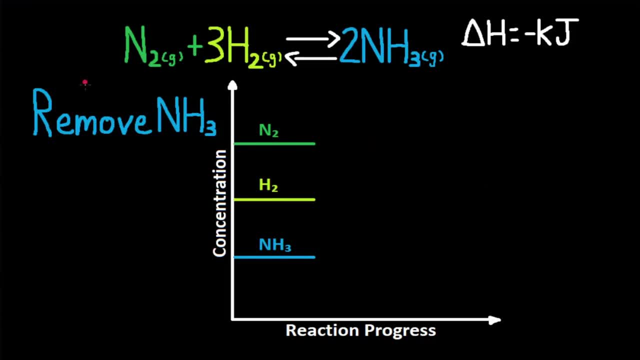 If NH3 is removed, describe the effect on the graph. Point at what is being removed. so this is a shift right. A shift right points at the products, so the products increase, and it doesn't point at the reactants, so the reactants decrease. And now we just graph what we described. NH3 is removed, so NH3 decreases. NH3 is a product, so it will increase. however, it won't increase more than its initial amount. H2 is a reactant and reactants decrease, so H2 decreases. N2 is also a reactant, so it will decrease as well. Remember to keep in mind. 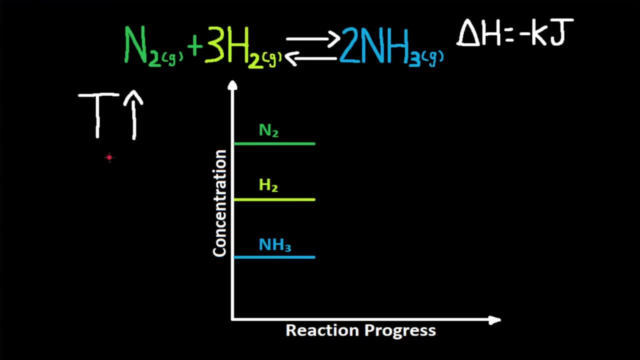 that coefficients determine how much it will increase If temperature is increased. describe the effect on the graph. This is an exothermic reaction because enthalpy is negative, so heat can be treated as a product. Temperature increases- don't point at what is being increased, so this is a shift left. Shift left points at. 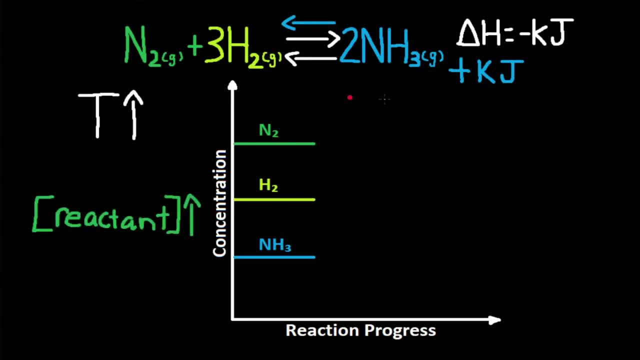 the reactants, so the reactants increase. and it doesn't point at the products, so the products decrease. For temperature changes, we just graph what the shift does: N2 is a reactant and reactants increase, so N2 will increase. H3 is a product, so NH3 decreases. 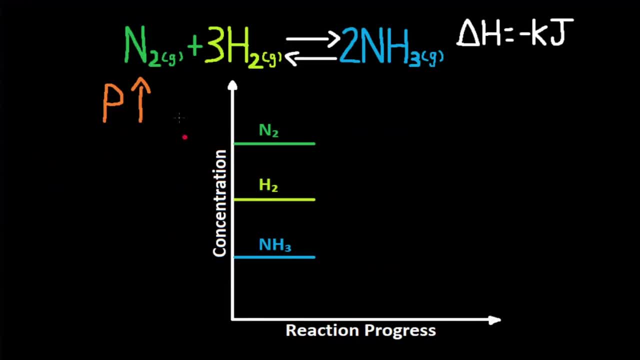 If pressure increases. describe the effect on the graph For pressure changes, we need to count the total gas moles on both sides. On the reactant side we have 1 from N2 and 3 from H2, so we have 4 in total. On the product side we have 2 from NH3, so we have 2.. When pressure increases point at the smaller number to reduce the extra pressure. A shift right points at the product, so the products increase in concentration, and it doesn't point at the reactants, so the reactants decrease. Now we just graph what we described. So since pressure increases, everything increases. first, N2 increases, H2 increases and NH3. 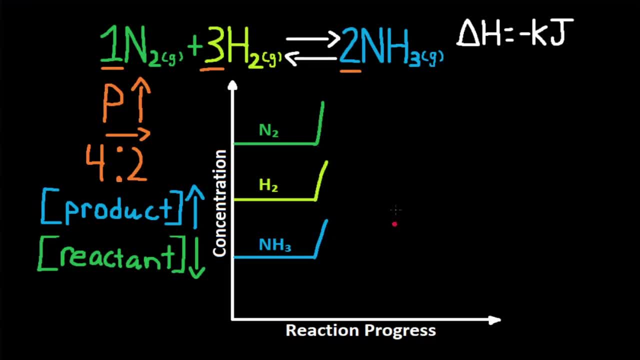 increases. If pressure decreased, everything would decrease first. Now we just graph the effect of the shift. So N2 is a reactant and reactants decrease, so N2 decreases. H2 is also a reactant, so it will decrease. is a product and products increase, so industry increases some more. Let's try this practice. 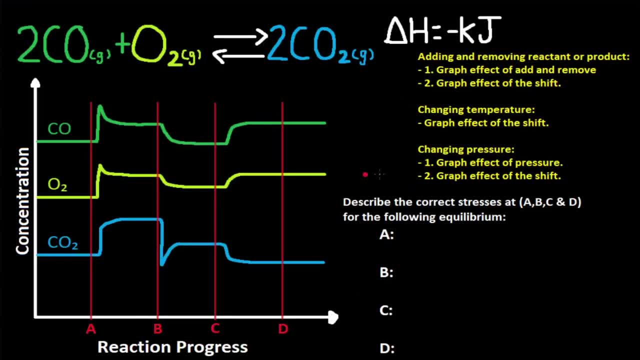 problem. In yellow are tips to help guide you. You can pause this video and do this yourself or work along with me. Describe the correct stresses at A, B, C and D for the following equilibrium: So at A, everything is increasing first, so this has to be a pressure change. 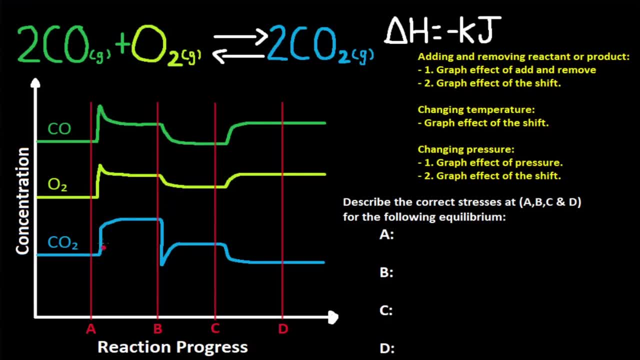 Pressure causes everything to increase or decrease first. Since everything is increasing, this means pressure is increasing. and let's confirm if pressure is actually increasing. So for pressure changes we need to compare the total gas moles on the reactant side and the total gas moles on the 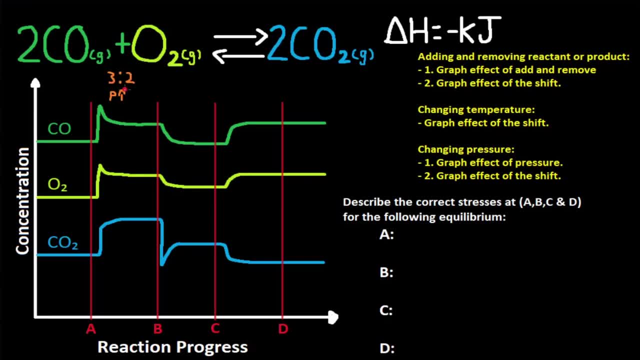 product side 2, 1,, so 3, and just 2.. When pressure increases, point at the smaller number. so this is a shift right. A shift right increases the products and decreases the reactants. So the correct stress at A is increasing pressure. At B we see that CO is decreasing and O2 is decreasing and the CO2 is. 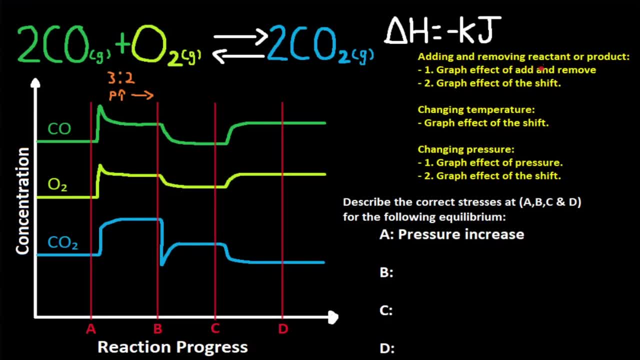 decreasing. So at B we see that CO is decreasing and O2 is decreasing and the CO2 is decreasing And then it's increasing. This has to be adding and removing a reactant or product and it's clear that CO2 is being removed. So when CO2 is removed, point at what is being removed. so this is a shift. 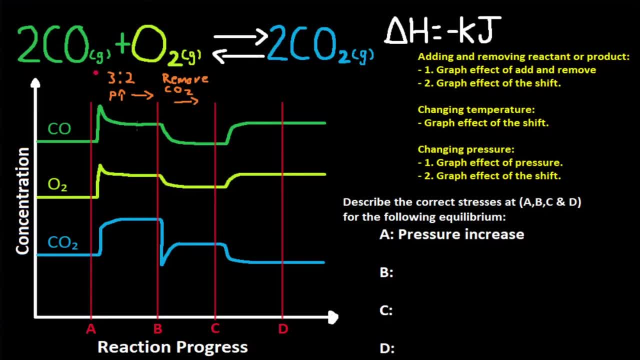 right- Shift right increases products and decreases reactants. Products should increase and reactants should decrease. So the correct stress at B, CO2 is removed. At C, CO is increasing, O2 is increasing and CO2 is decreasing. This is most likely a change in temperature, since it is just